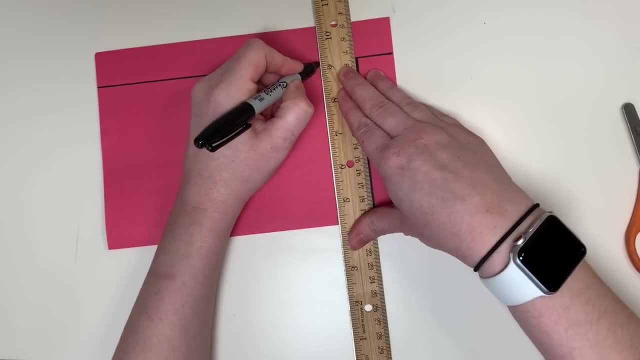 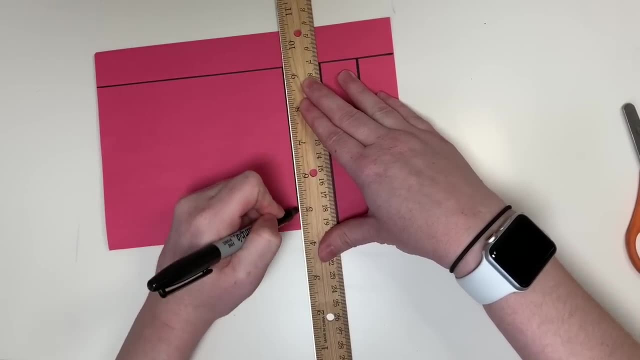 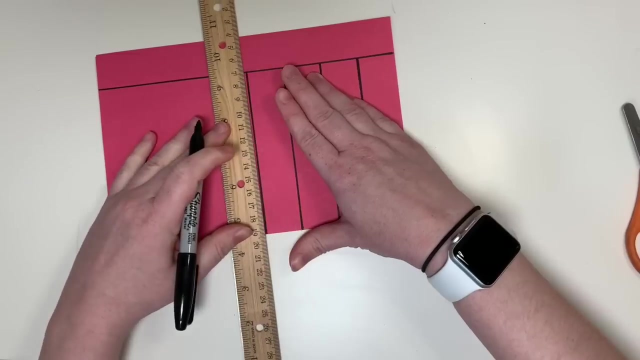 just match up your ruler or whatever you're using to measure and fill in as many as you can. I suggest tracing a little bit more slowly than you're used to, because you want it to be your absolute best and it will really help when we are weaving. 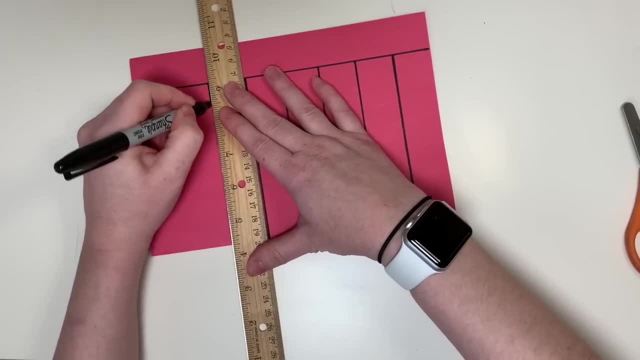 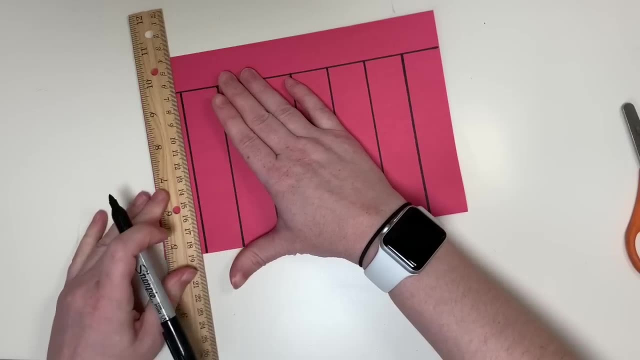 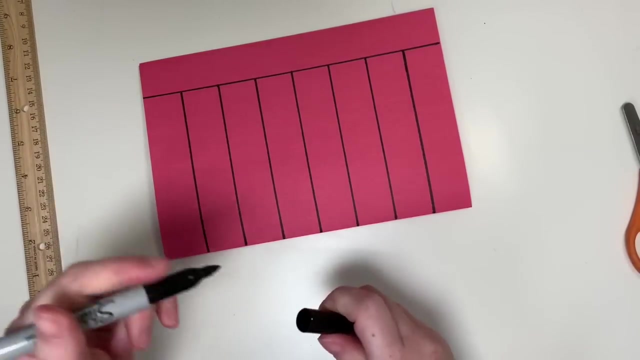 Now, because of the size of my paper, I'm not going to be able to fit the ruler in perfectly for my last one, so it's up to you. if you end up with enough room for a small line, go for it, but I'm going to leave it just the way it is, and now I'm going to keep it closed. 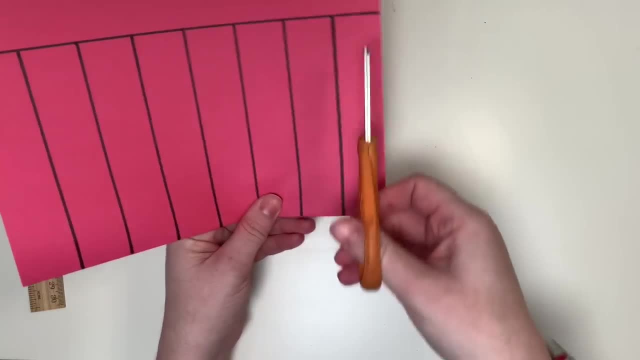 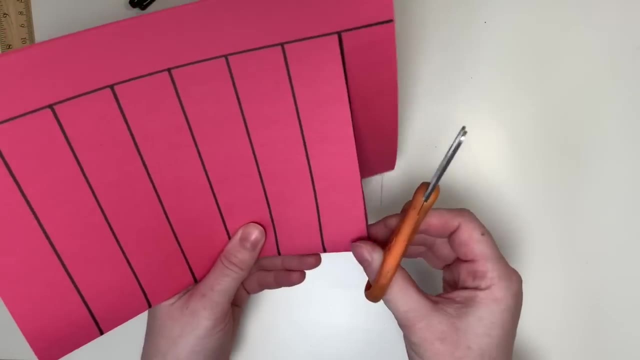 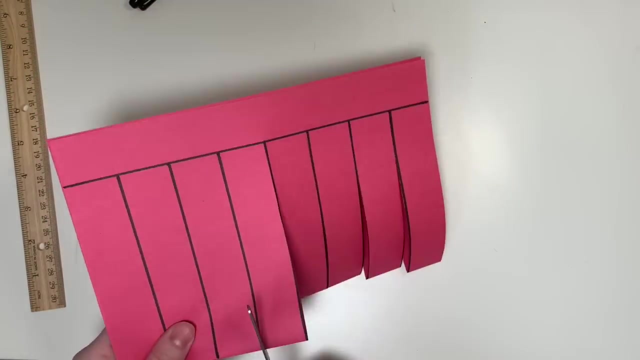 but I'm going to grab my scissors and I'm going to cut up these lines and stop at the top of that paper. reliable lines- that is what these are going to be. you're going to want to hold your paper so that it doesn't shift. do the best you can. 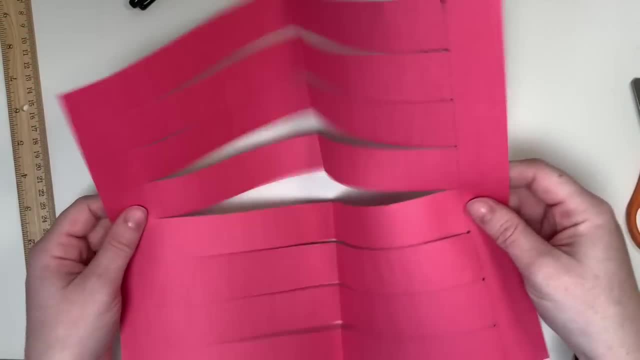 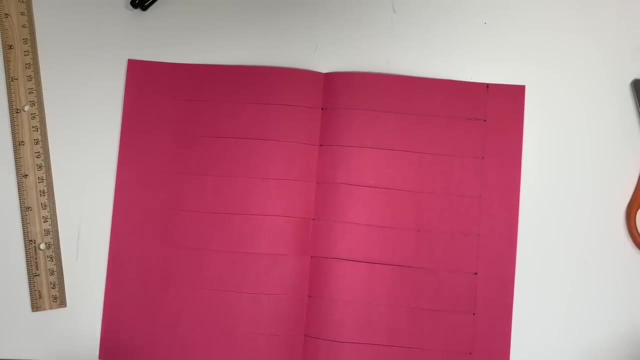 And now my loom is finished. when I open it up, I have all of these different pieces that I can pull apart, but they're still attached on the ends. Now I need something to weave with, and that's where i'm going to need my second piece of paper. 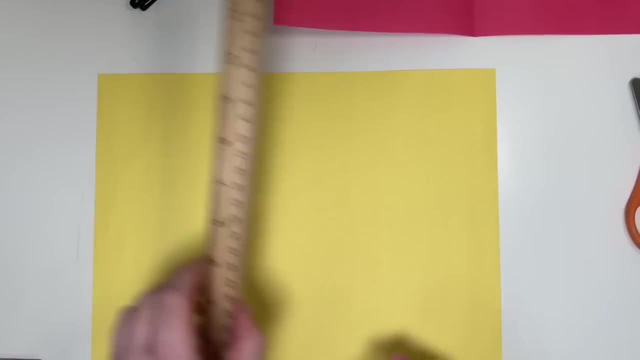 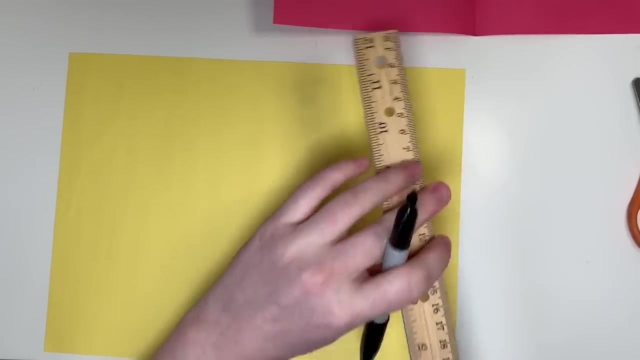 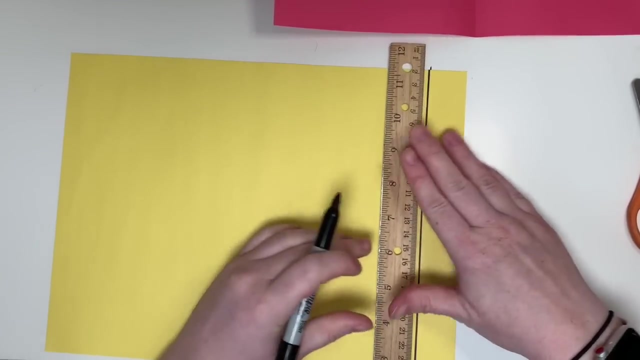 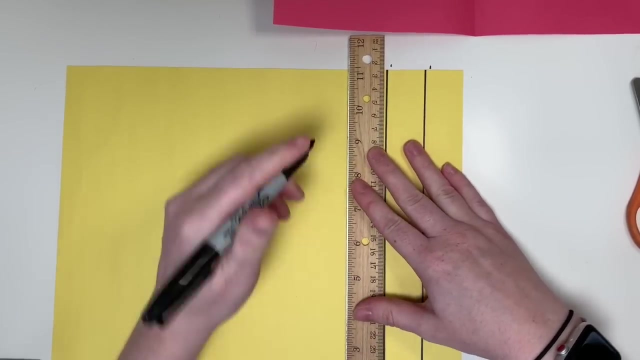 again, you can use any piece of paper that you want, but just do the best that you can. and to make these into even strips, I'm gonna use my ruler trick again, where I line it up to the edge. now, weaving reminds me an awful lot of science, because you can change the paper, you can change the size, you can really. 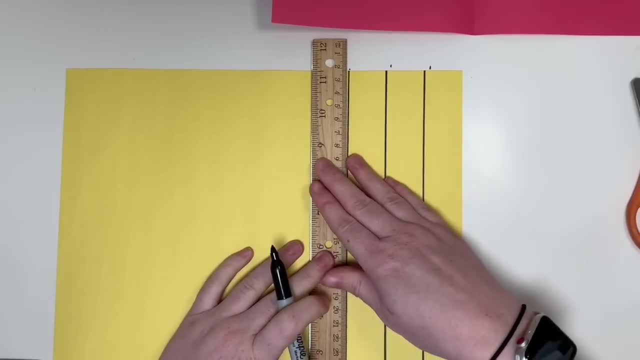 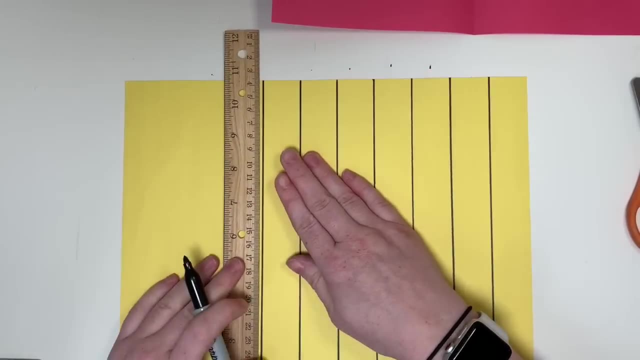 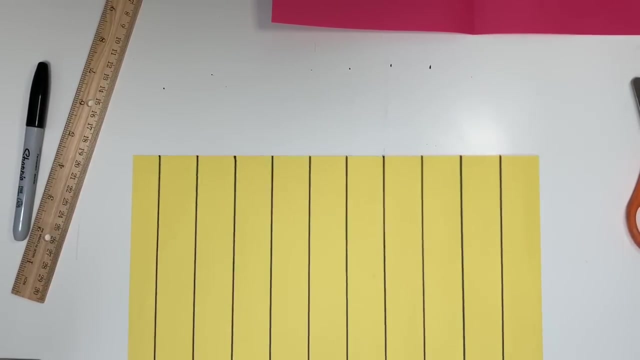 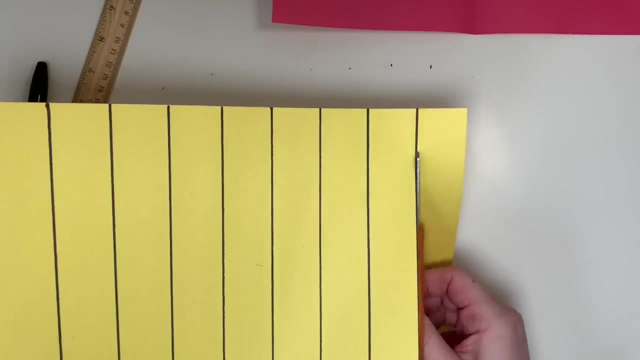 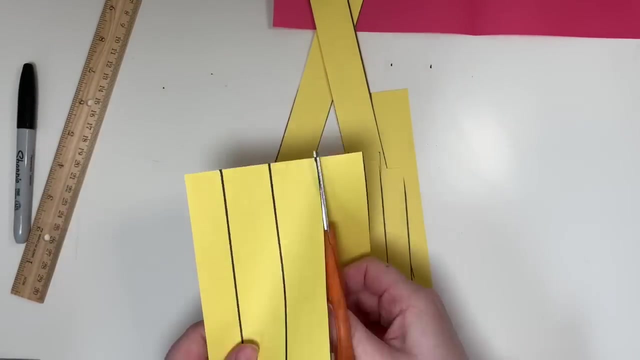 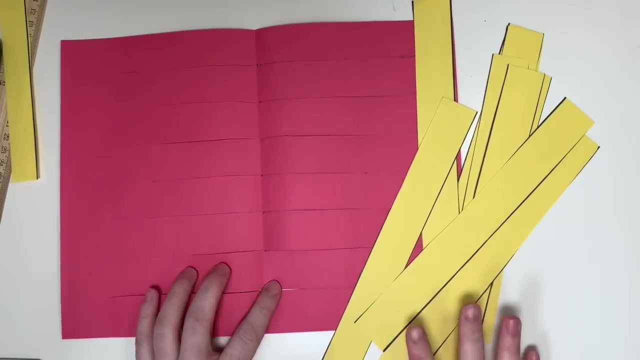 experiment and see how yours turns out differently. and every time you make it different you learn something new. can you guess what I'm gonna do next? I'm gonna cut these out. do the best that you can, because you don't want jagged edges. all right, it's time to weave the basic.